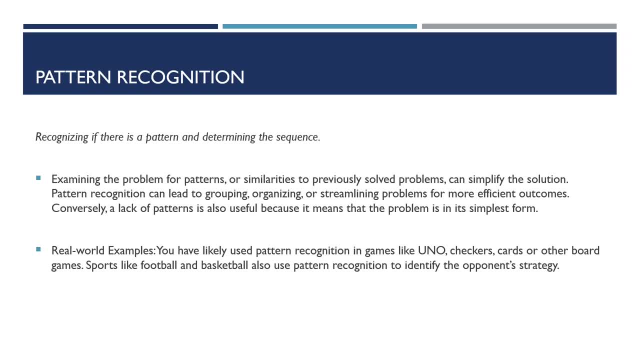 services, Yet they always have similar features. They always have a button to create a new message, some type of folder arranging system, some type of search system so you can search through emails. They're similarities or patterns. There are patterns that exist in the problem of sending an email and they're 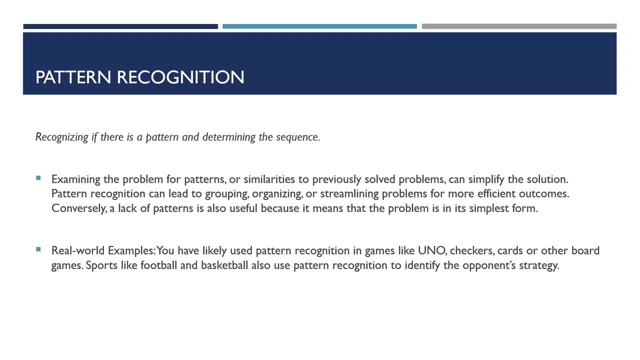 solved in different ways, using different user interfaces and giving a different user experience. If we look at them, we can draw out the patterns or the key things that need to exist and integrate them into our own solution for that particular problem. So pattern recognition can lead to the grouping or 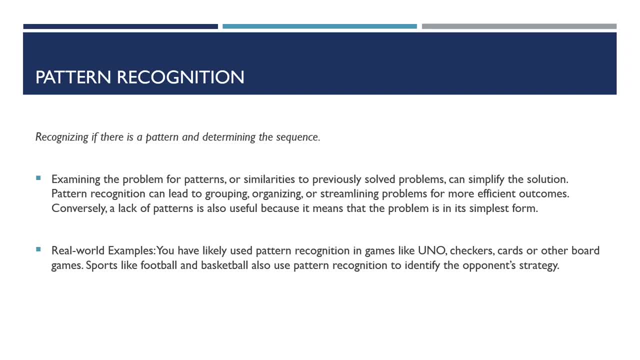 organizing or streamlining of problems for more efficient outcomes. On the other hand, if you can't find any patterns or there's no grouping or no similarities, then that's not a bad thing either. It means the problem is probably in its simplest form, Potentially So. 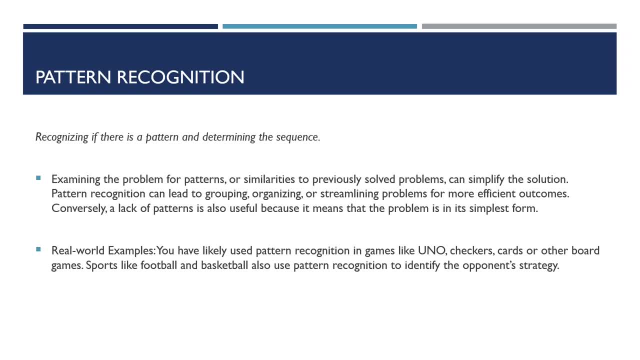 you've seen patterns heaps and heaps of times. If you ever played a board game, there's a pattern in that. If you played card games, there's patterns, There's strategies, there's tactics. If you watch the sport, or cricket or football- the teams have 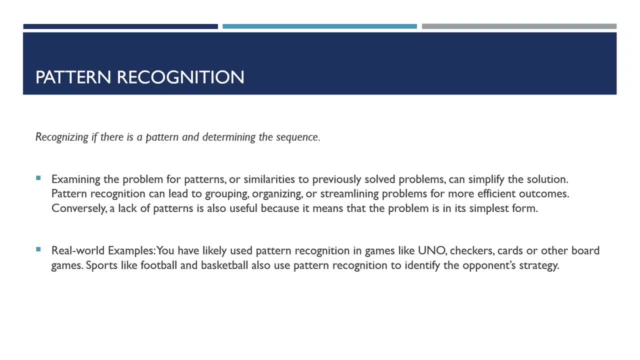 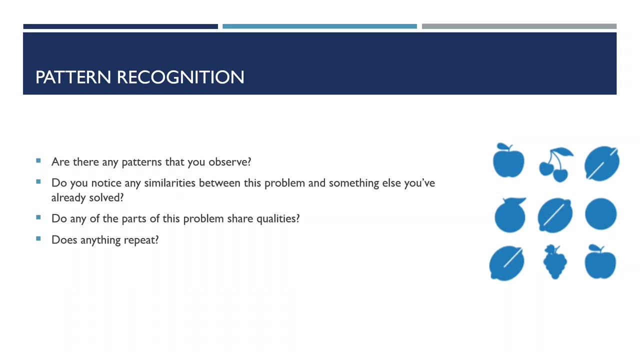 certain plays or certain ways of acting in the game, or tactics or strategy that people will show and their pattern. and if the opposition works out the patterns then they can counter them. So when we're doing pattern recognition, the key questions we want to ask are: Are there any patterns you observe? Do you notice? 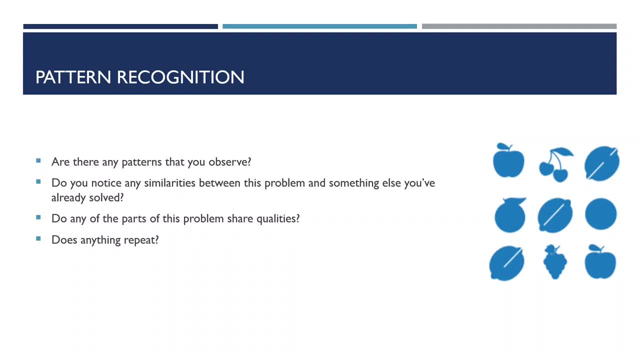 any similarities between the problem and any thing else similar that's been solved? Do any of the parts of the problem seem similar to each other? For example, you have one form people enter personal information. in another form Do information and another form where they enter some other type of information. 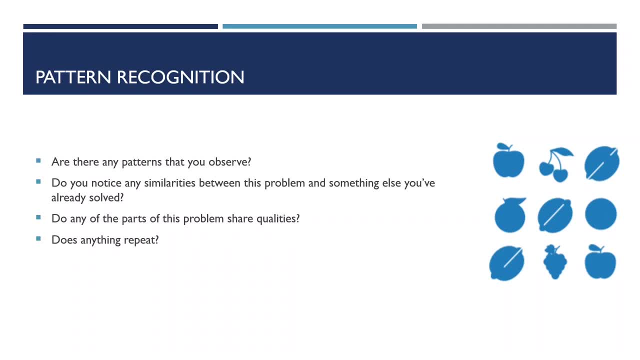 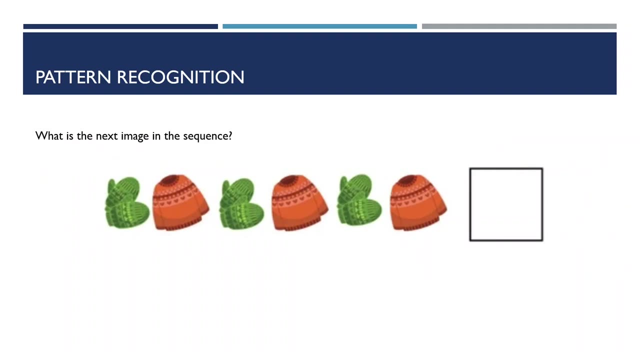 well, they've got two forms there, so maybe the technology to use both of them is quite similar and all you need to do is change the question. you're looking for things that repeat, so let's just do a little bit of pattern recognition as an exercise. what's the next image in the sequence? okay, so the next image in the 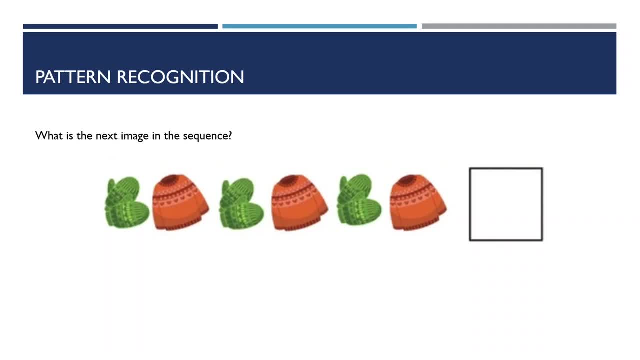 sequence. how well, what is it? it's probably the, the green minutes. but how do you know? because you've seen there's a pattern. it's a repeating pattern. here goes green orange, green orange, green orange. so, logically, the next thing is green. so we found a pattern. okay, let's try something a little more difficult. 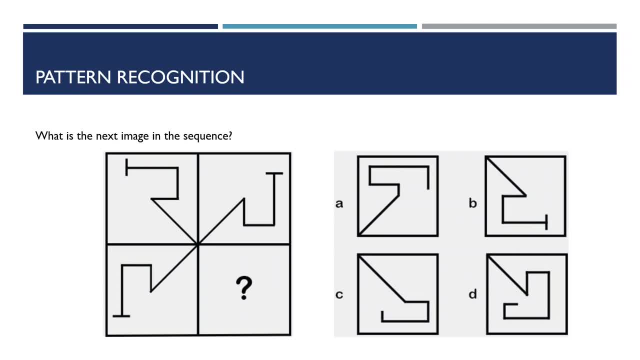 what's the next image in the sequence? I'll give you a minute or so, or 30 seconds to think about it. okay, so have you thought about solving this problem? what patterns can you see? well, I can see that in each instance, radiating from the center outwards there. 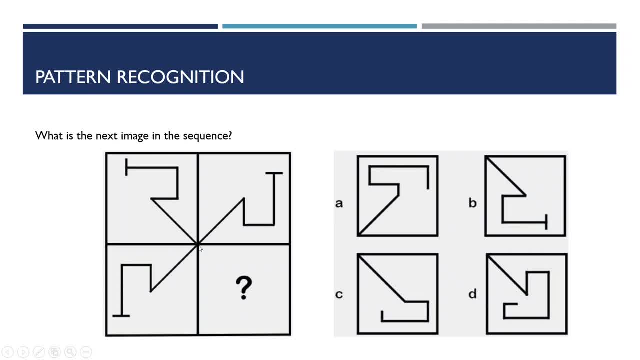 is a diagonal line, you, so this one probably has a diagonal line coming out, so automatically I know it's really going to be B or D or C, so it's not gonna be A. now what happens when you go out? so here you go out and you turn to the right and you go out and 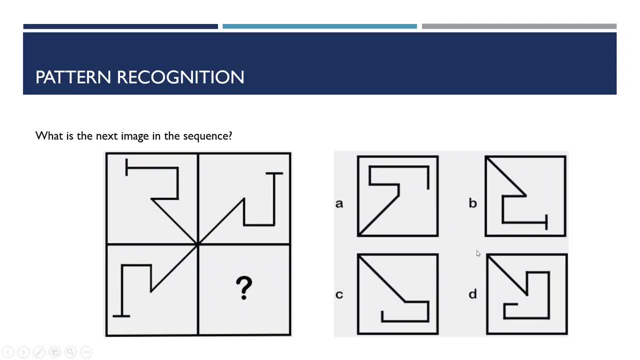 you turn to the right and you go out and you turn to the right so I need to go out and turns right so I go out and I turn right. so it could be B. go out and I turn to the left, so it can't be D and I go and turn to the left so it can't be C. 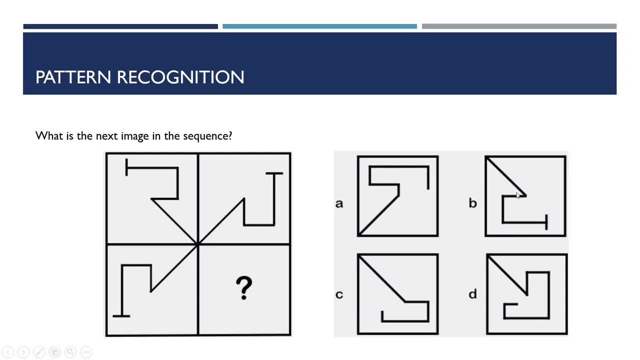 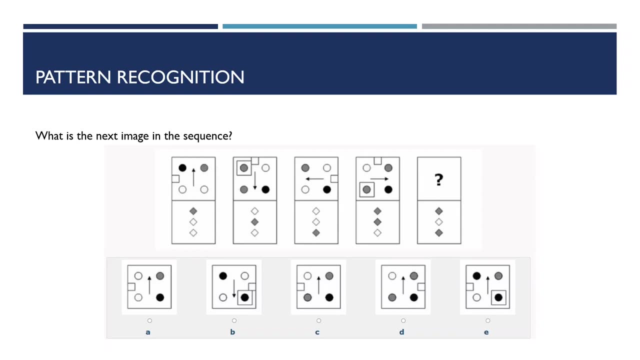 so automatically I'm thinking B is the answer and I'm pretty sure B is the answer. so B is the answer. so by observing patterns we found, so I'll just leave you with one more to conclude this section on pattern recognition: what is the solution to this problem? what is the missing image in the 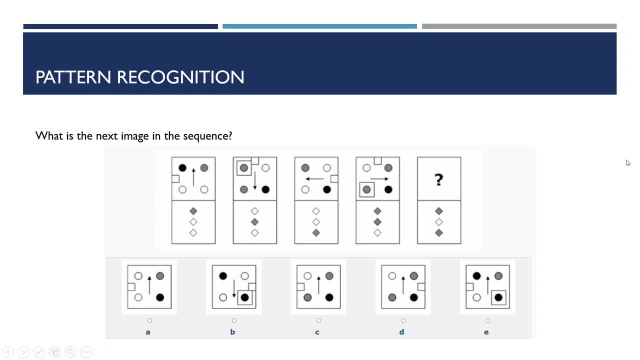 sequence. okay, so I'm gonna. I'm reveal the answer now. so if you still want to solve it by yourself, you should pause the video and have a crack. otherwise I'm just going to go through and talk through how you might solve this problem. so we're looking for patterns, so let's have a 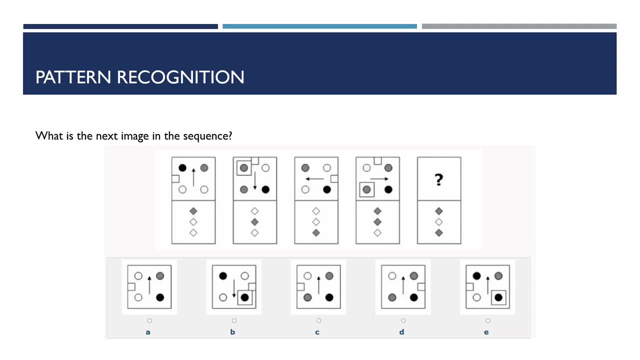 think about what's going on. so let's start with the arrows. so the sequence for the arrows is up instead of it really going upwards, so actually it's up governments on that. So let's start with the arrows down left right. so up down left right. so the next arrow is probably going to be pointing up. 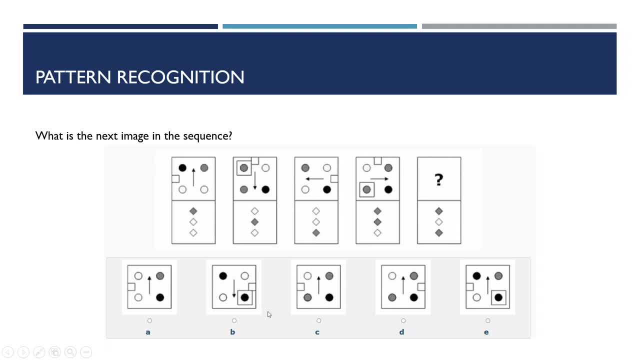 so it means it's not B, so what else can we think about it? so let's think about this little notch on the edge. so what's the pattern here? well, it goes left top, right top. so if it's following a pattern, it's going to go left top. 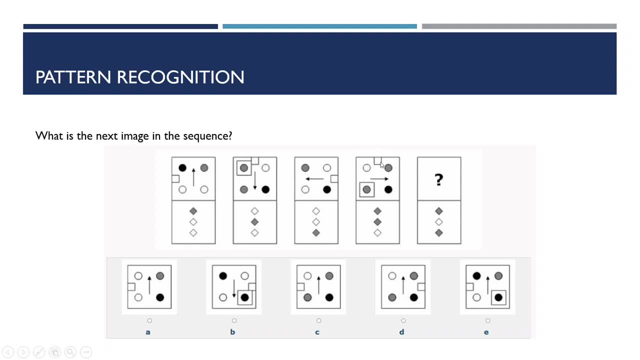 right and then back, and so to the top and then back to the left. so we're expecting the notch to be on the left. so if the notch is on the left, that means it's got to be either A. it's got to either be C or it has to be E. 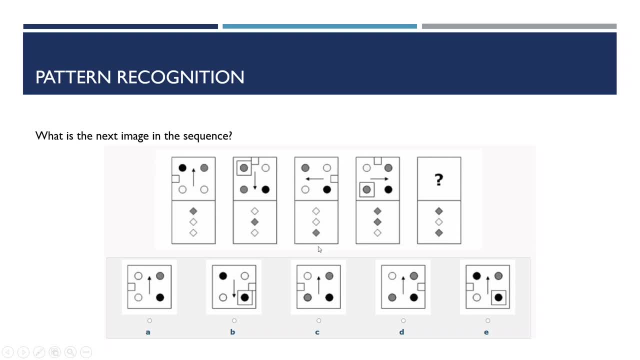 okay, let's have a look at anything else that's noticeably as a feature here. well, this is a square that appears around, so there's no square, square, no square, square, no square. so we want something that has no square in it. so that brings us down to A or C. 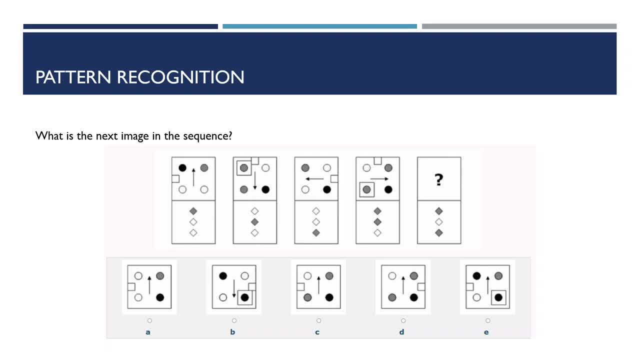 so it's A or C. so how are we going to differentiate between A and C? maybe there's something to do with the colors of the dots, because that's the only thing that's left left. so we took the color klarino. we put like this along: 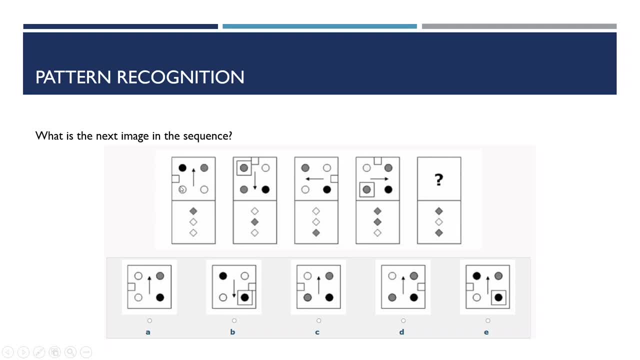 back to the beginning. so, whatever the color, income in A was like black, so we got all of our blue values. so now, if we look at black, let's use this for blue again, with nothing white. so now let's look at black. if we look at light, white or two colors, so let's talk about white and with a bright color, then white's 0 and 2 and 2 might Men's count, that is 7 and 1 right now.